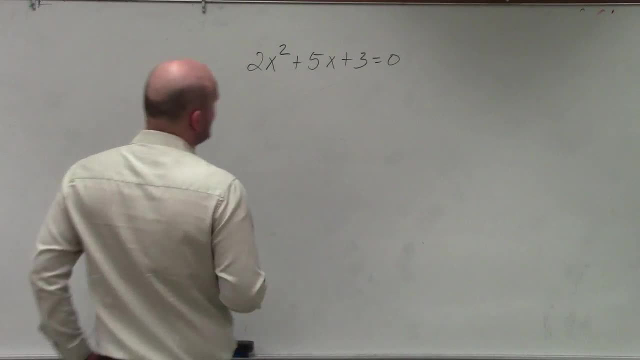 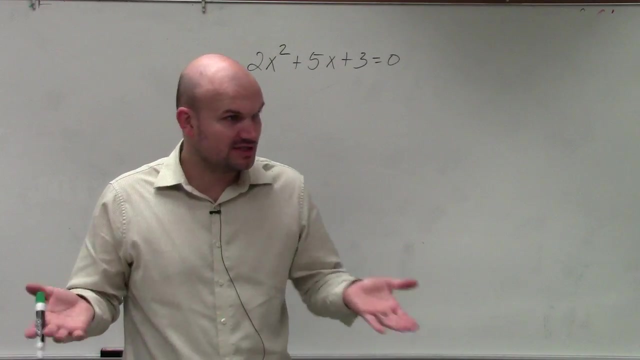 In this example. ladies and gentlemen, if we're doing Descartes' Rule of Science, all Descartes' Rule of Science tells us is the number of possible rational zeros right. It just tells us the number of possible- I'm sorry, the number of possible real positive, real negative and imaginary zeros. 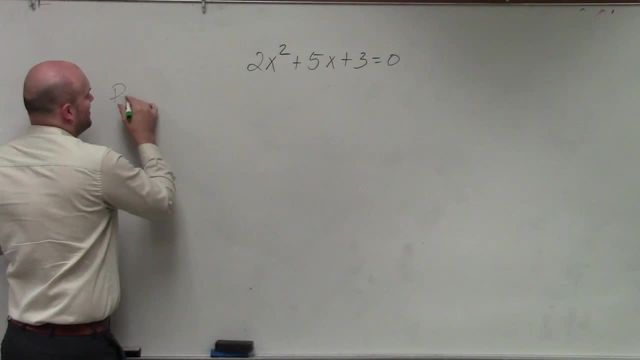 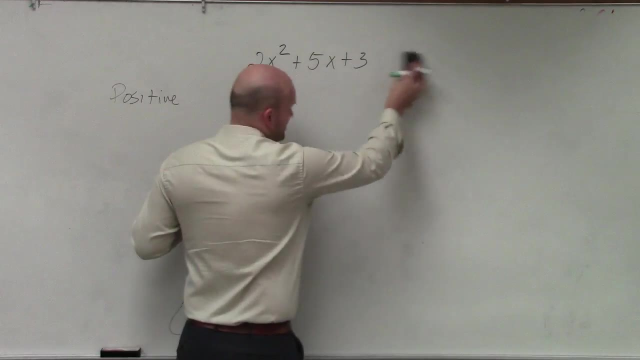 So if you guys go ahead and look at this to determine the number of positive, first of all I know this is an equation sine equal to zero, because this is a different type of problem. Usually a lot of times you're going to have it set up as a function. 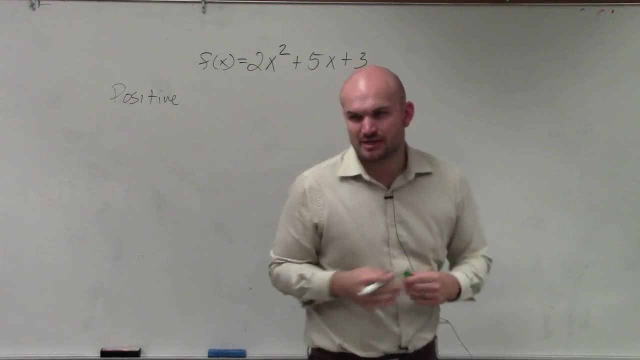 So, for my instructional purposes, I'm not going to set it equal to zero, I'm going to set it equal to f of x. I'm going to relate this as a function Because, remember, I told you I gave different kind of examples. 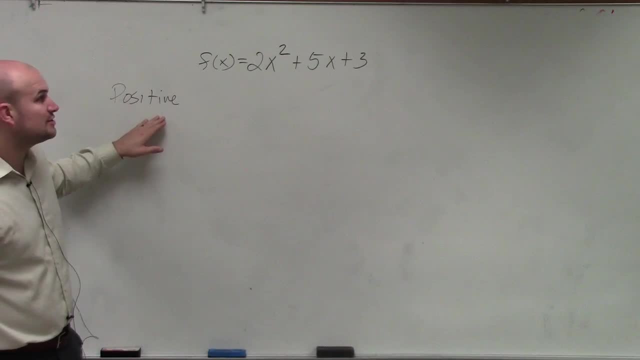 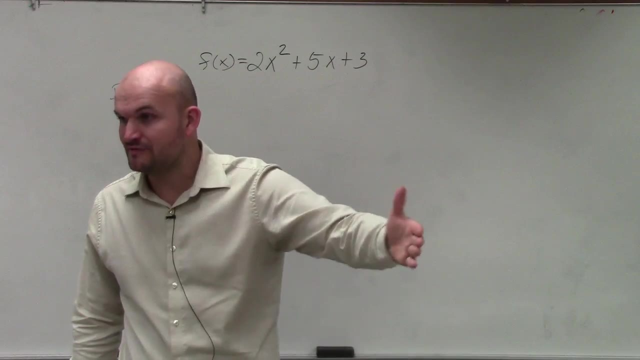 So, anyways, to find the number of positive, real solutions, all you're going to do is count the number of sine changes. Anytime you have a term that's positive and the next term is negative, that's a sine change. Anytime you go from a negative term to a positive term, that's a sine change. 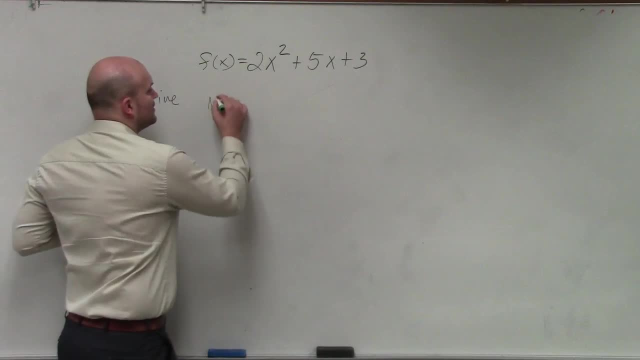 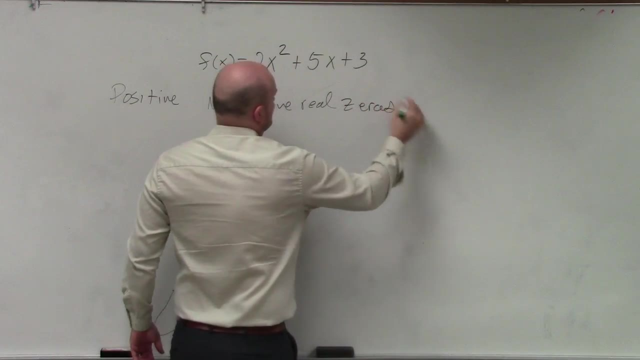 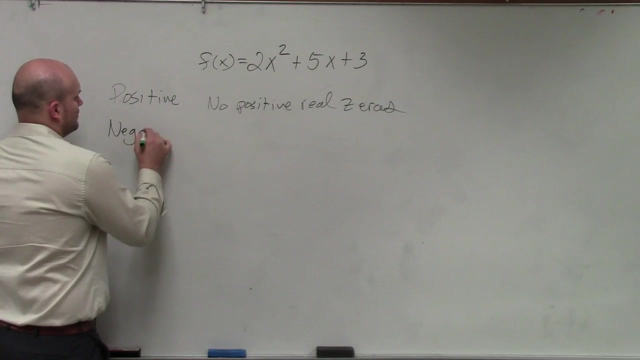 So do you guys see any sine changes here? No, So guess what? There's no positive real zeros. Okay, No positive real zeros. To find the negative, what we need to do is figure out what is f of negative x. 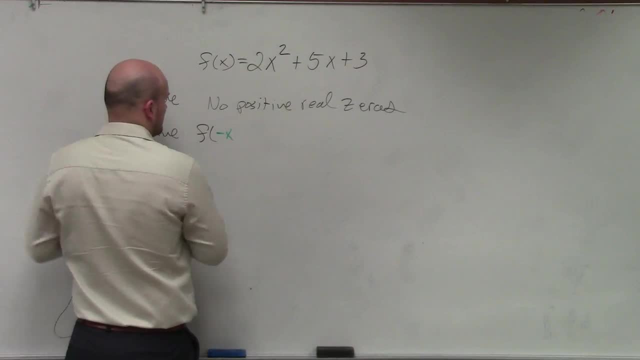 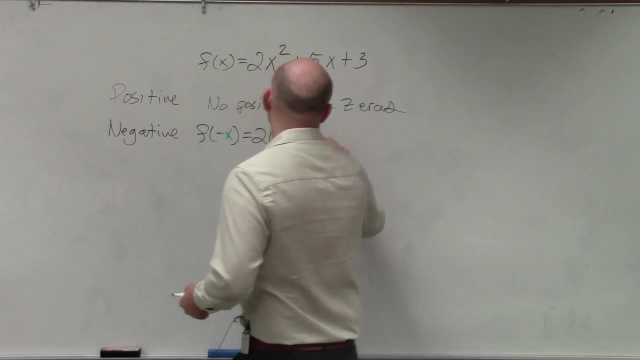 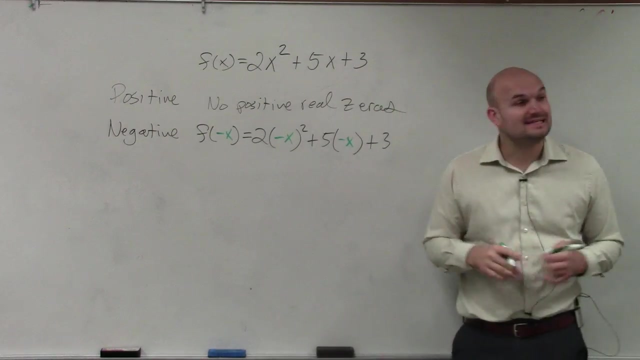 Well, we'll go and see f of negative x. So that gives you 2 times negative x squared plus 5 times negative x plus 3.. Anytime you have a negative term raised to an even power, that's always going to be positive. 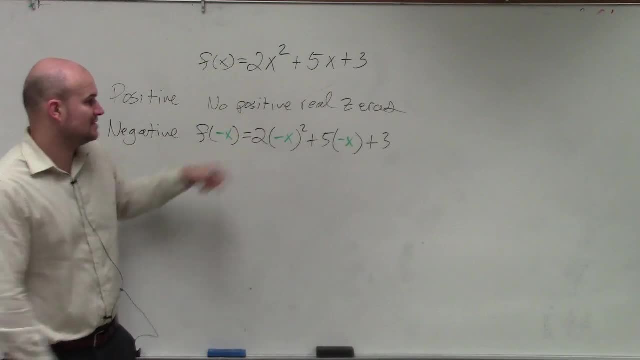 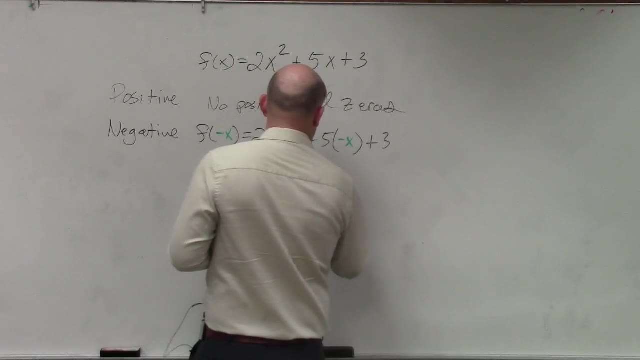 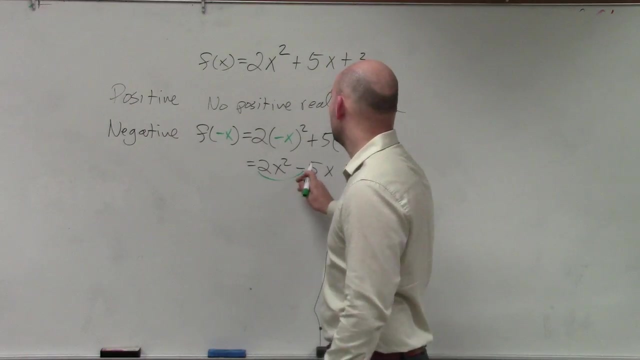 So negative x squared is positive x squared. Positive x squared times 2 is 2x squared. Negative x times 5 is a negative 5x, And then we have plus 3.. So, yes, exactly as Drew said, We can now count the number of terms or number of sine changes. 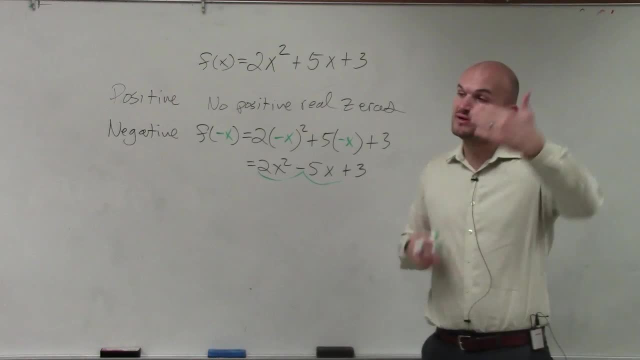 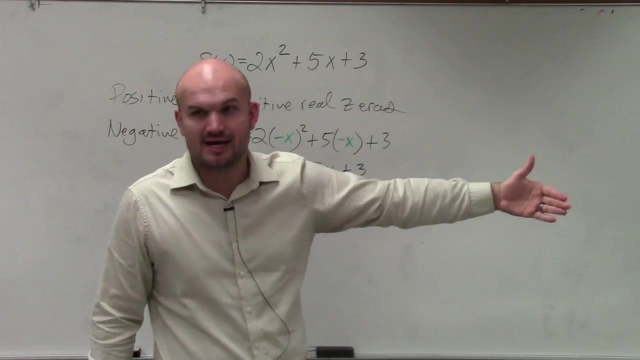 We now have 2.. But please remember, Descartes' rule of sine says it's the number of sine changes minus an even number. Well, think of the most common even number would be 2.. I always just like to subtract 2 as much as I can. 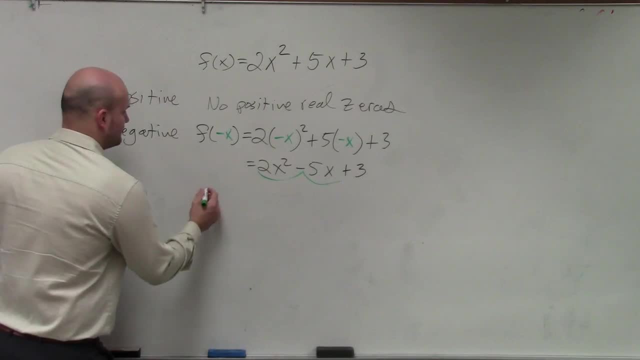 So, if I have, So, for the number of negative, we're going to have 2 or 0. Because 2 minus 2, subtracting of an even number, 2 minus 2 is 0.. Negative Real zeros. 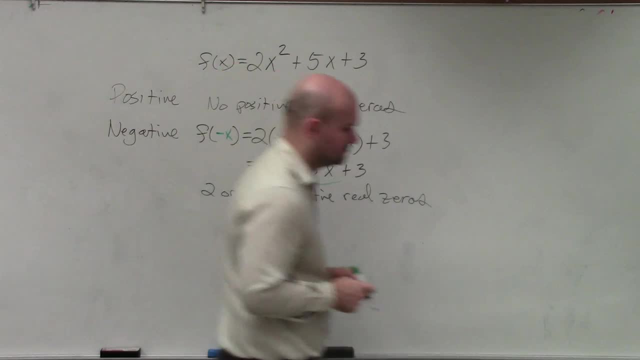 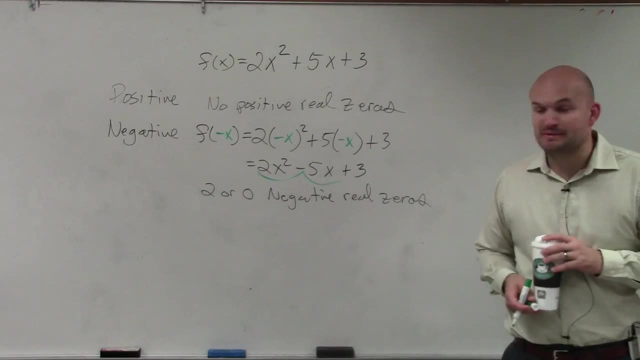 Yes, That part kind of confuses me. So what if the sine changes, Or the sine changes 4 to 5 times? Then the number would be 5, 3, 1.. 5 minus 2 is 3.. 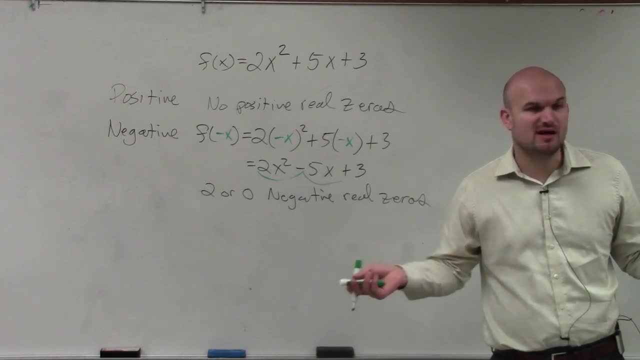 3 minus 2 is 1.. I can't subtract 2 from 1 and still have a positive number, So then I stop at 1.. But yes, always just keep on subtracting 2 until you can't go any further. 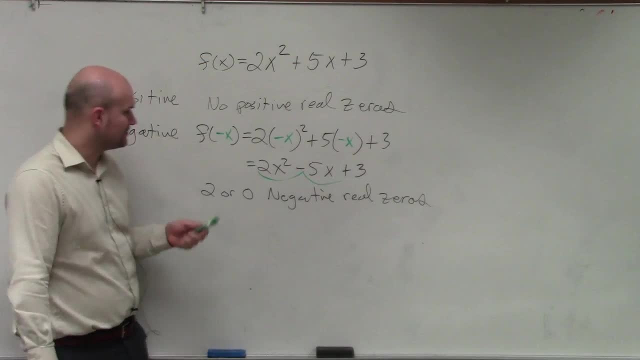 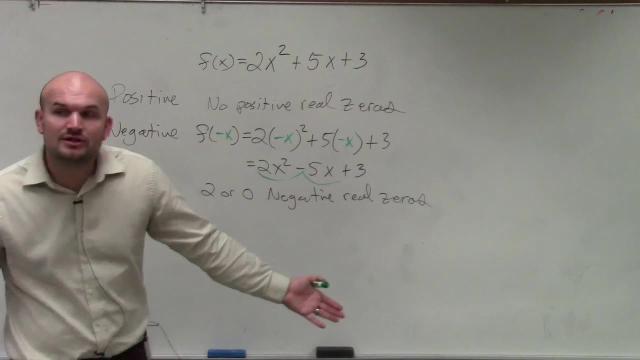 Okay, You're either going to end up at 1 or 0, basically, So you have 2 or 0 negative solutions. Now I have 2 options here for the negative right. So what if I ask? What if the question, though, on the test was: hey, how many complex are there? 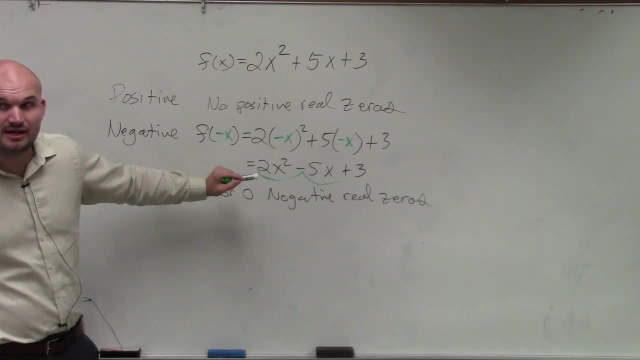 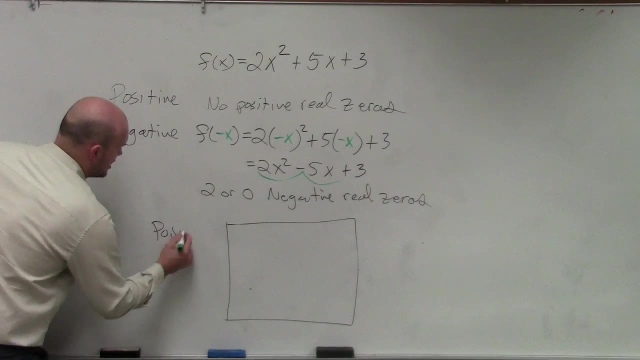 Well, this tells you they're a real positive, real negative. It doesn't really tell you the complex. So we have to create a chart, Or at least I like to create a chart, And my chart consists of positive, Negative. 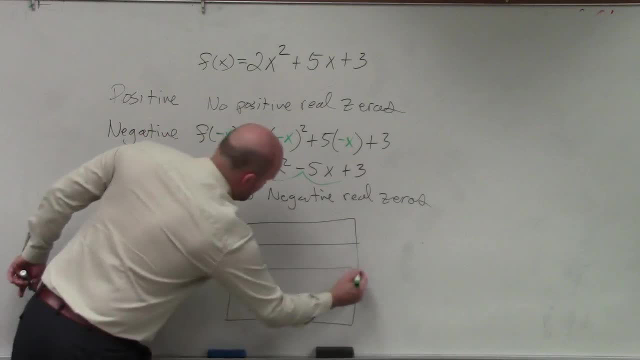 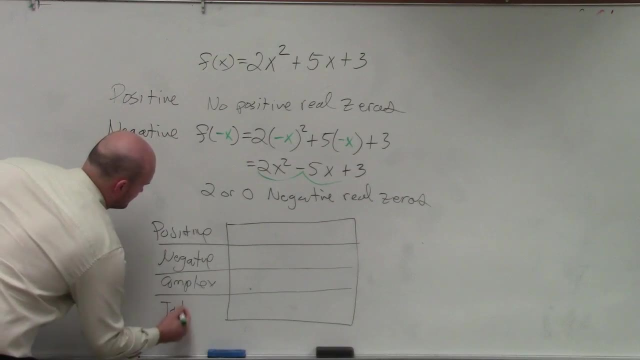 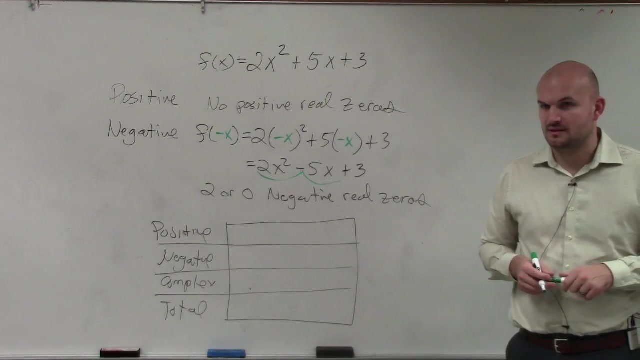 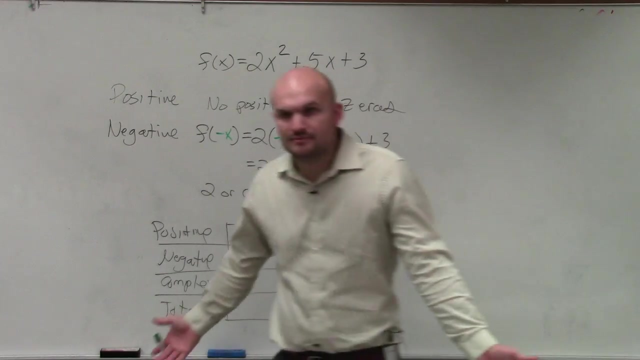 Plus 2.. Bless you. Complex. And the total, Yes, Yes, Okay, So, for the number of positive, Well, actually, first of all, we can do a couple of these: How many total solutions do we have? That is based on the what. 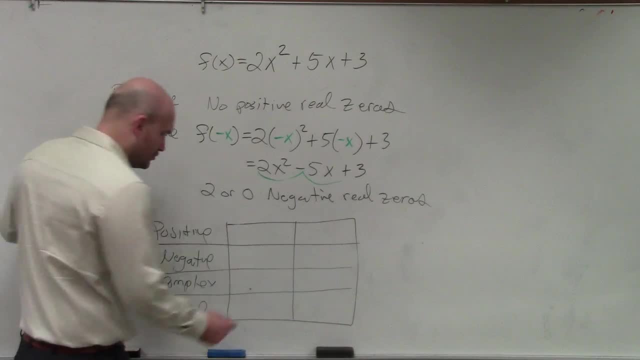 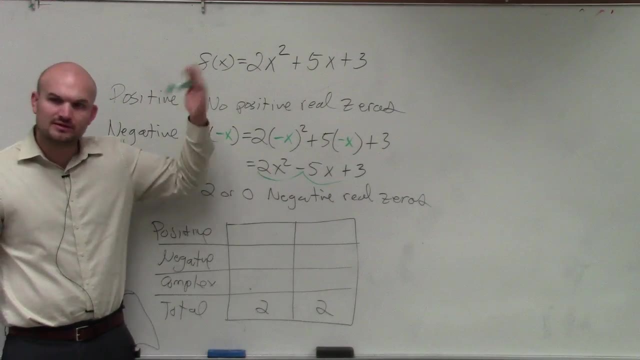 Degree. So the total number of solutions is 2.. How many turning points would there be in this graph FYI? 1. It's always. 2.. It's always n minus 1, right, Where the degree minus 1.. 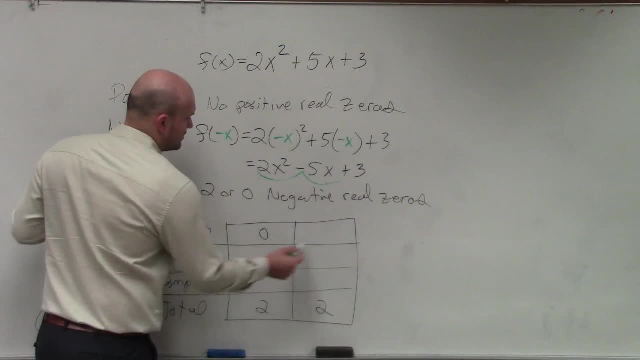 All right. So the number of positive. We said there's no positive real zeros, So we'd have 0.. For the negative, we said there's 2 or 0. It's one or the other. That's why I have those two columns. 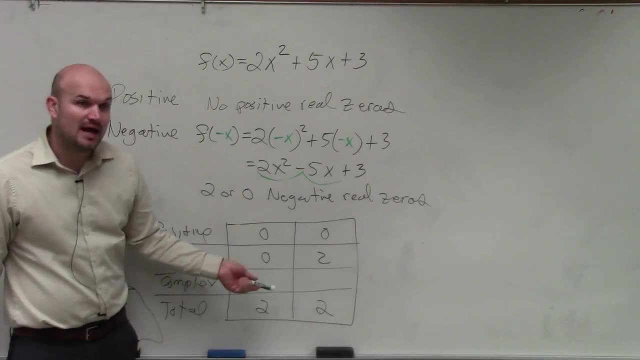 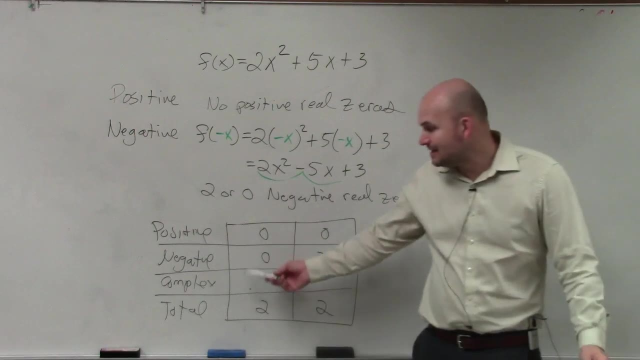 So it's 0 or 2.. So, to find the number of complex. Well, ladies and gentlemen, if I have 0 positive, 0 positive real, 0 positive negative, then how many complex are there? How many complex do I have to have to satisfy my two solutions? 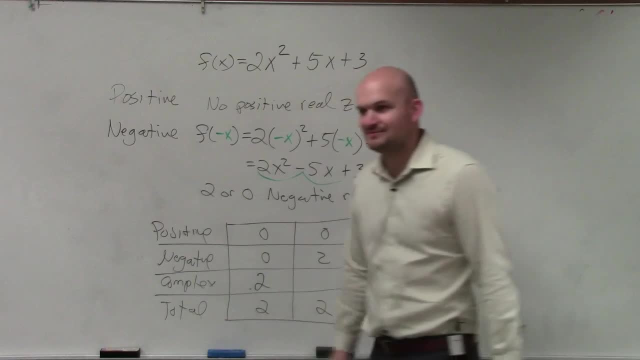 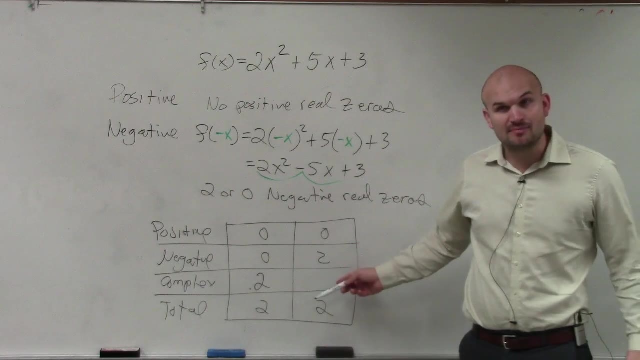 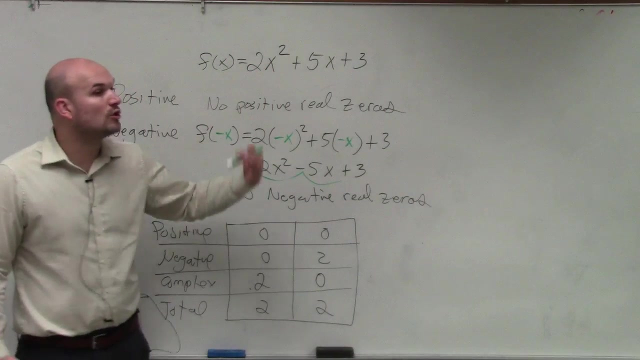 2. 2. Right, If I have 0 positive, 0 negative, I'm sorry. 0 positive, 2 negative. how many complex do I need? 0.. So the number of possible complex solutions is going to be 2 or 0.. 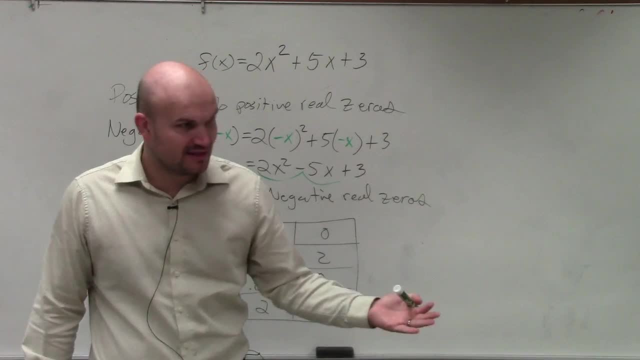 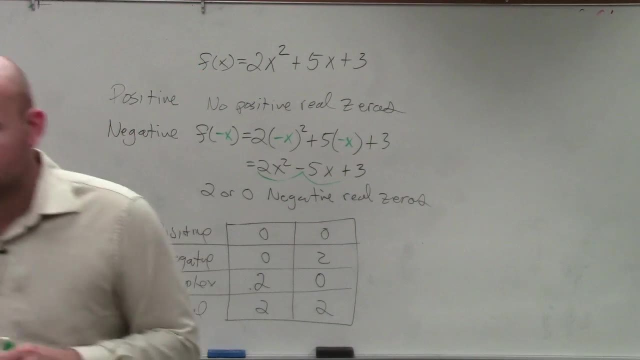 Okay, Again, decartical science does not tell you which one it is, Which one is which, It just tells you what your possibilities are. Okay, Yes, Phil. 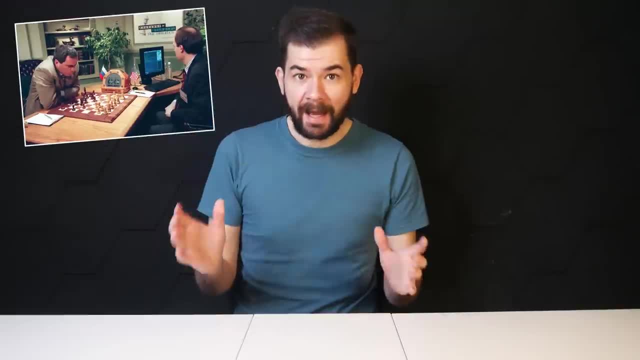 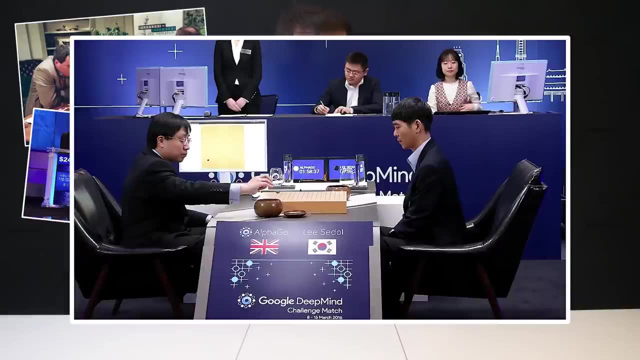 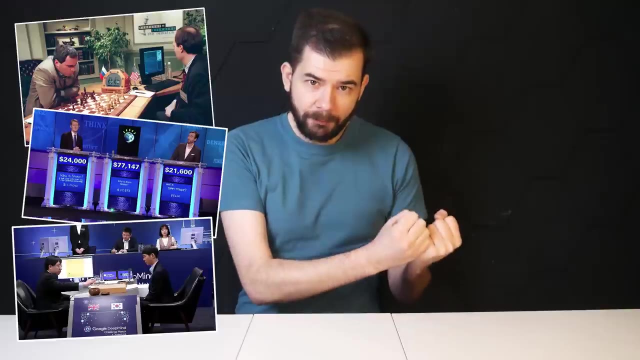 In 1997, computer Deep Blue beat the highest-rated player at chess. 2011,. computer Watson beat champion players of Jeopardy 2016,. the game Go fell to the computer AlphaGo. But these are just games. What about a demonstration of practical problem-solving? 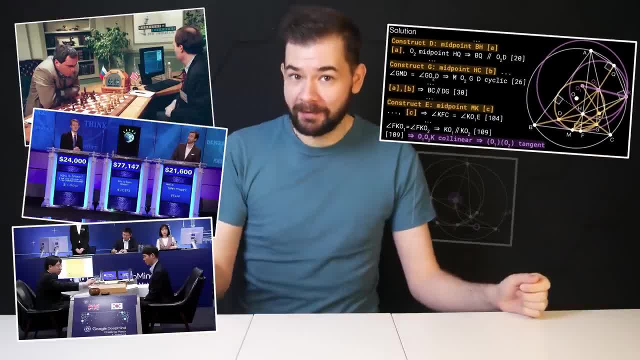 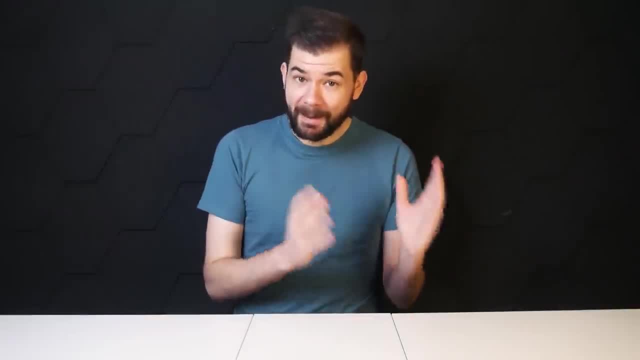 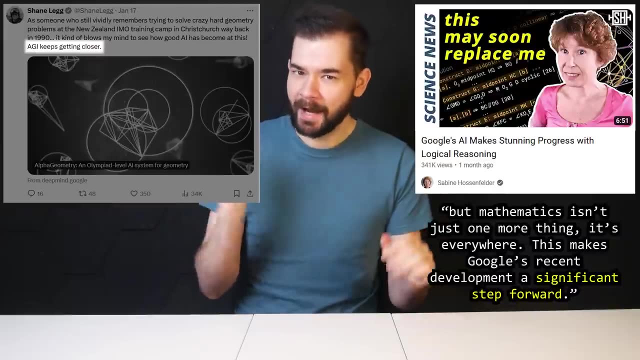 Enter AlphaGeometry, an AI developed by DeepMind that can solve Olympiad-level geometry problems, outperforming the average human participant. This has been heralded as a massive leap in AI reasoning and a step towards artificial general intelligence. But is it? I'll give my thoughts in this video. 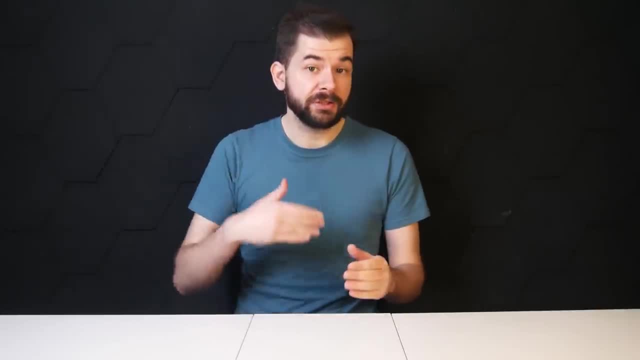 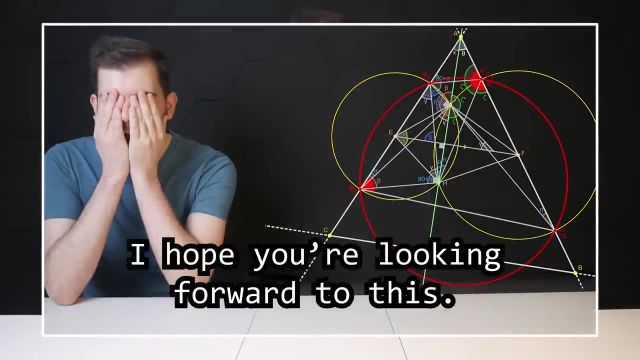 Firstly, how does it work? No coverage I've seen actually goes into any detail of AlphaGeometry's solutions. I went through them and it was so painful. I feel it's only right that I inflict that experience on others. but trust me that pain is worth it as it will help us in the second half. 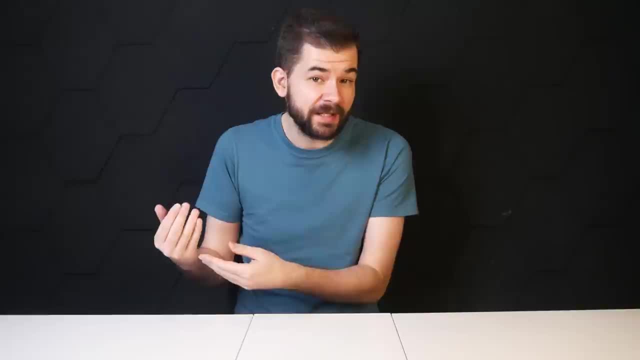 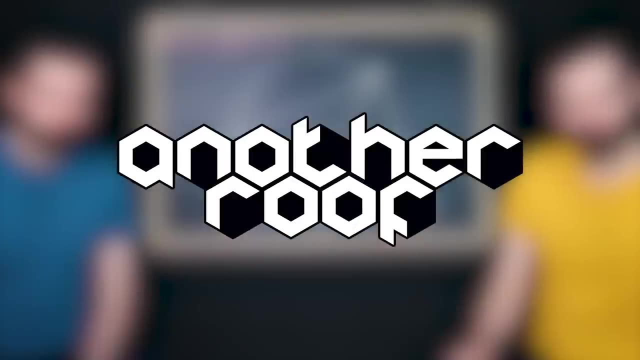 of this video where we discuss whether this is actually a step forward in reasoning or not. I hope you enjoy this video and I'll see you in the next one. First a brief look at how AlphaGeometry works and then a deep dive into one of the Olympiad. 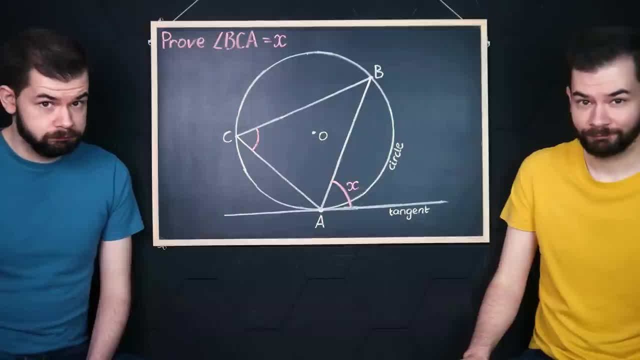 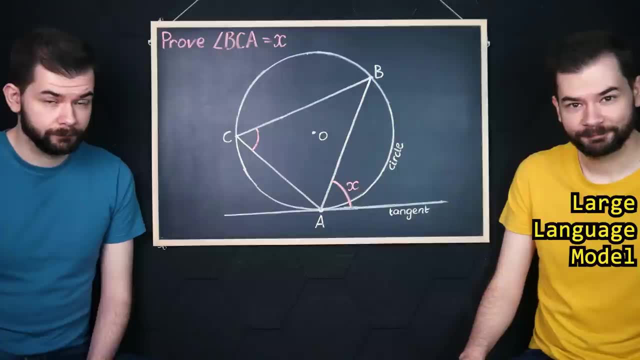 problems it solved. It is made up of two systems and I'll demonstrate what it might look like if it tries to prove this well-known result. The first system is a language model akin to a refined and specific use ChatGPT. I suggest ideas like plot the midpoint of this line or draw this.